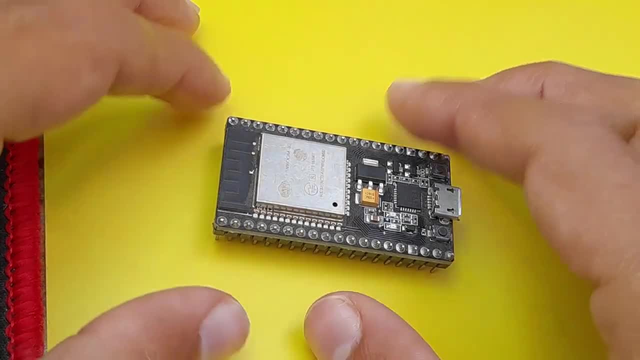 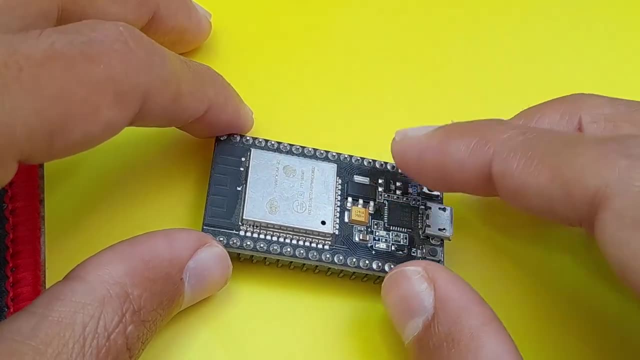 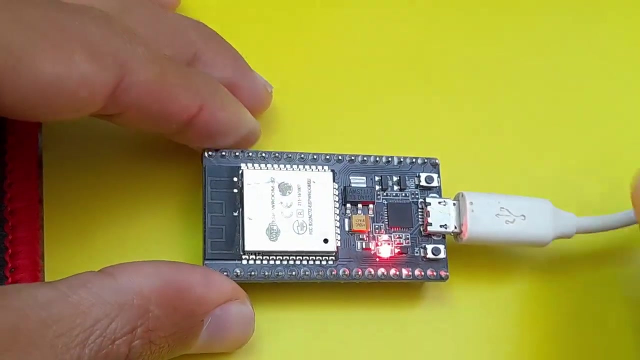 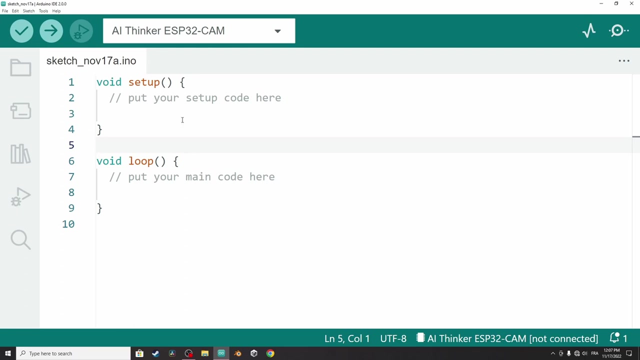 So, as I said at the beginning of the video, the ESP32 board comes with the built-in Bluetooth module that you could use. First we have to plug in the USB cable so that we can program it with the Arduino IDE. Then let's open up the Arduino IDE. Here we have an empty sketch. So first of 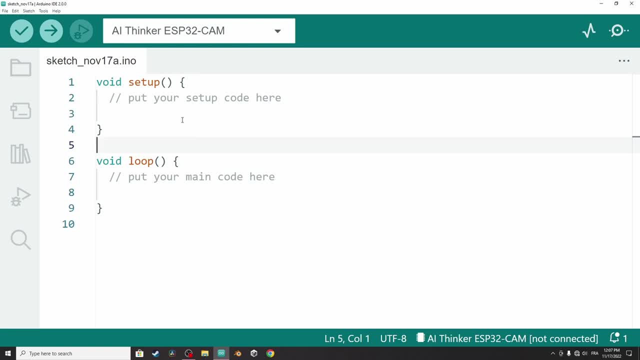 all we have to include a library, which is called the Bluetooth serial. that allows you to use the Bluetooth feature And you don't have to install this library, it is built-in. You simply need to include it using hash, then include and the name of the library. 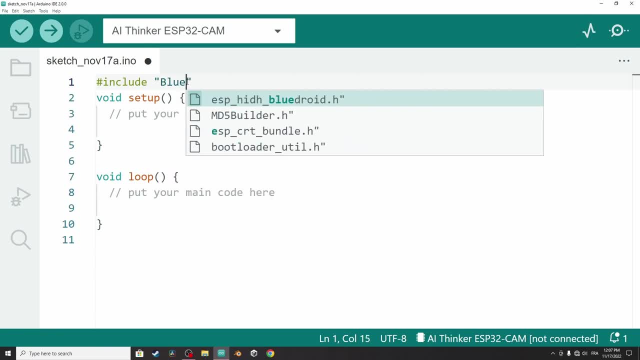 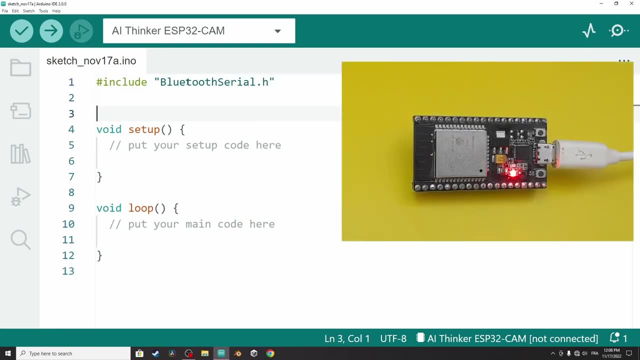 in these double quotes, which is Bluetooth serial. Then we add h because it's a library. After that, we can create a Bluetooth serial object that represents the Bluetooth module of the ESP32 board using Bluetooth serial, And we can give it a name. You could call it whatever you want. I'm going to call it serialbt. 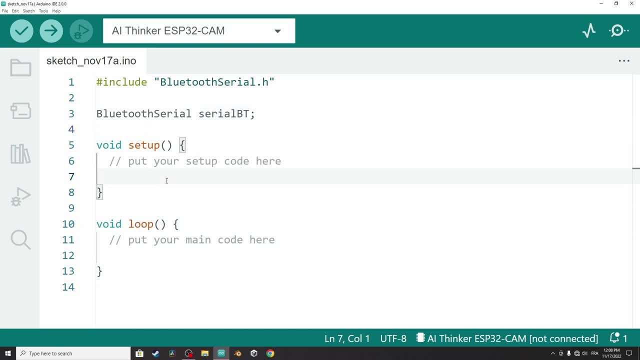 Then we have to enable it under the setup function using serialbt, which is the name of the object. Then begin: This takes a string in these double quotes And it's going to be the name of the device. So when you open up Bluetooth, 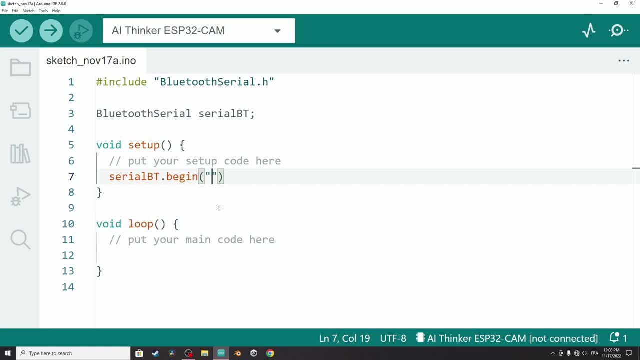 you will see the name of the Bluetooth module. For example, I'm going to call it ESP32-bt, And don't forget the semicolon. Then, under the loop function, we can check if we have received a command or some sort of message from Bluetooth, And to do that we can use an if statement. 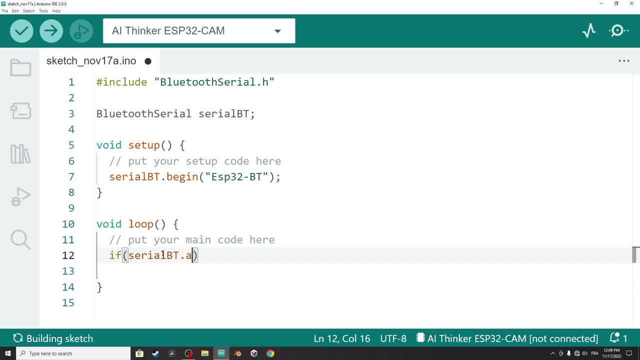 using, if serialbt available. So this is a built-in method. It's going to be true when we have a message that we can read, or a character. In such case we use serialbtread, And this is another method that returns the character that we read. 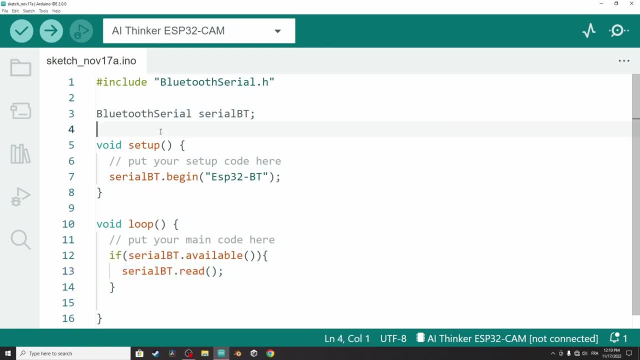 We can put it inside a variable. So let's go on top. The type is character or char. Let's call it cmd, Then we can assign the value to it using cmd="serialbtread". And that's pretty much it. Now you could use this command to control LEDs or. 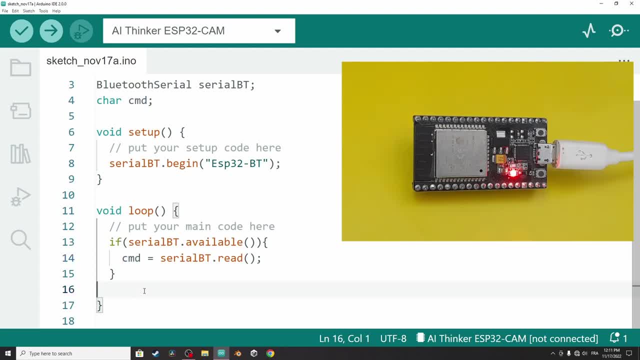 other devices that are connected to the ESP32 board. For example, let's turn on and off the built-in LED. So the ESP32 board comes with a blue LED that we can control And it is connected to the pin number 2.. I've talked about that in the first video. 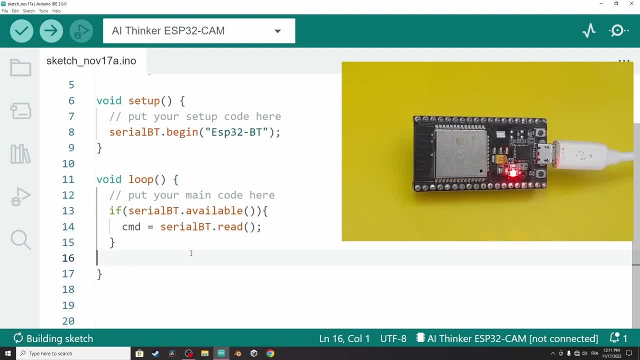 i've talked about that in the first video, in the first video. so let's add this logic: we can check if the command cmd equals, for example. 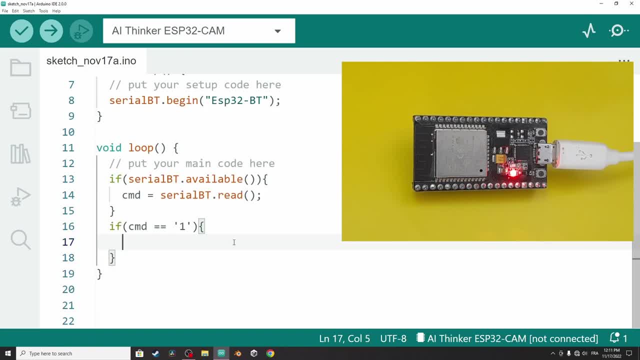 the character 1. in such case, we turn the LED on using digital write. this command takes the pin number, which is 2, and to turn it on we use high, and that outputs a voltage from the pin number 2 and turns the LED on. and with the same way we can check if the command equals 0 using if cmd. 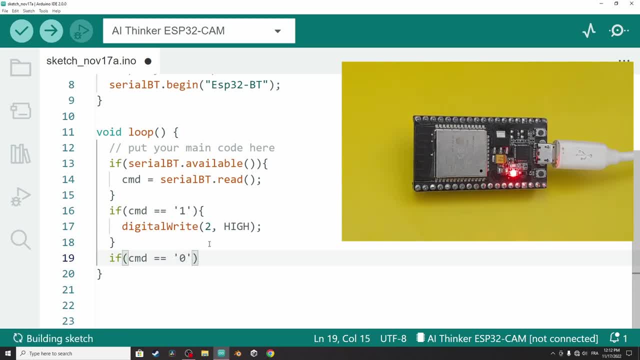 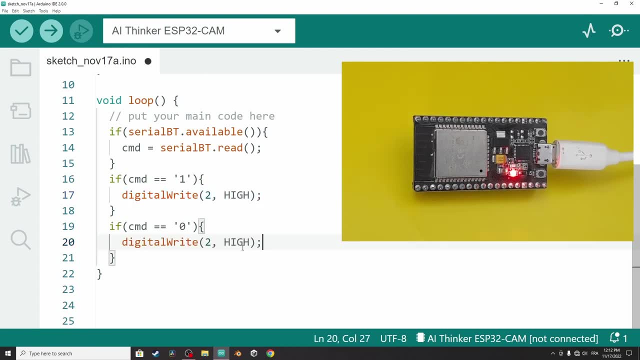 equals the value 0, then we could use digital write low. so I will just copy it and turn it on and paste it, and don't forget to change this to low. and last but not least, it is recommended to add a little bit of delay to the loop function because it is called so fast. we have to slow down. 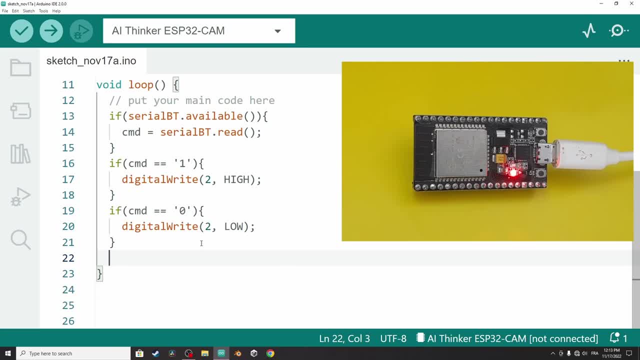 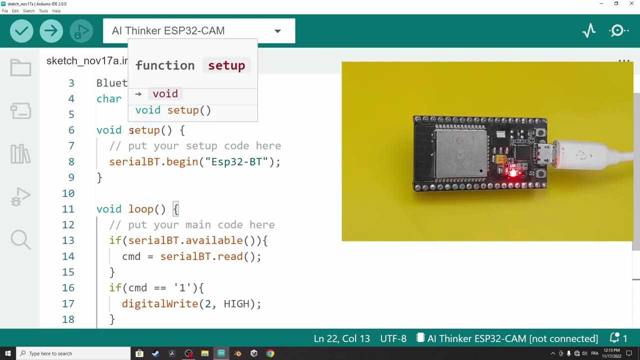 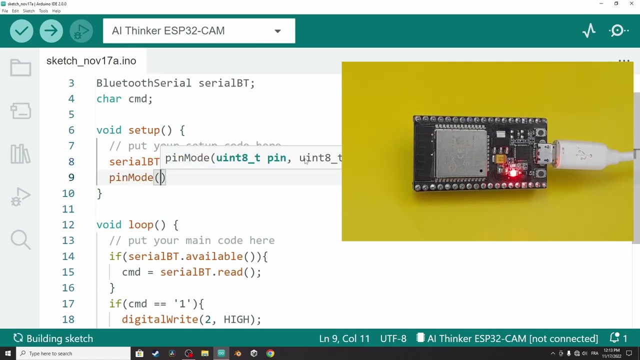 the program to smooth it using delay. so this method takes the number of milliseconds. I think 20 milliseconds is fine and that's pretty much it. but I think I forgot to add the pin mode under the setup function. we have to add pin mode. we give it the pin. 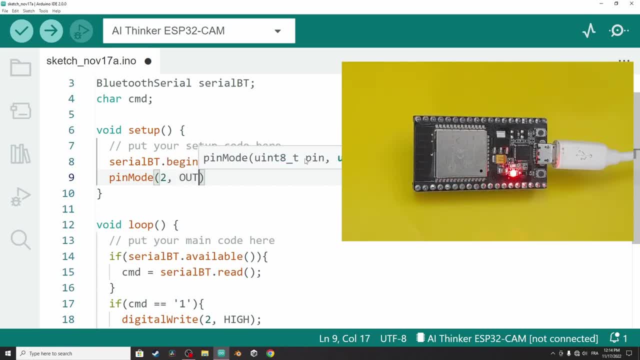 number 2 and the output keyword, because in some cases we have to use the pin as an input, for example, to read a value from a sensor like the temperature and the humidity. anyways, before we upload the code, we have to select the kind of board that we are going to be using for the 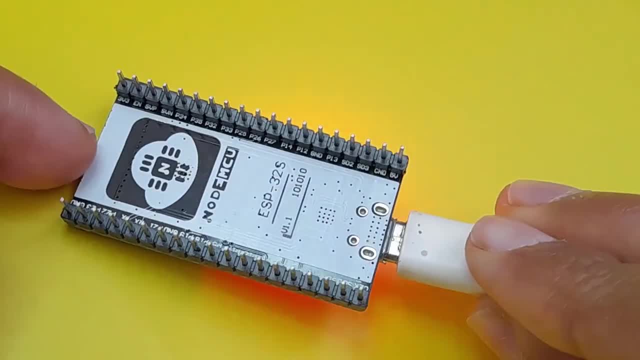 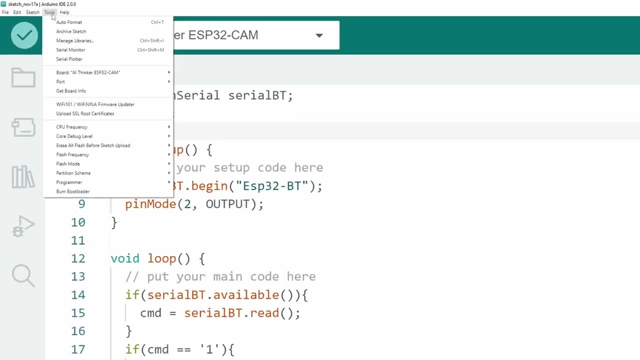 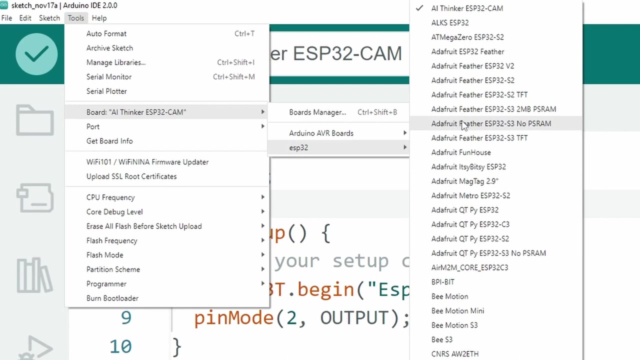 test, and then we have to select the kind of board that we are going to be using for the test. for me it is called NodeMCU ESP32S, and to do that you have to go to tools, then board. under here we have ESP32. of course you have to set up the Arduino IDE and install the ESP32 package. 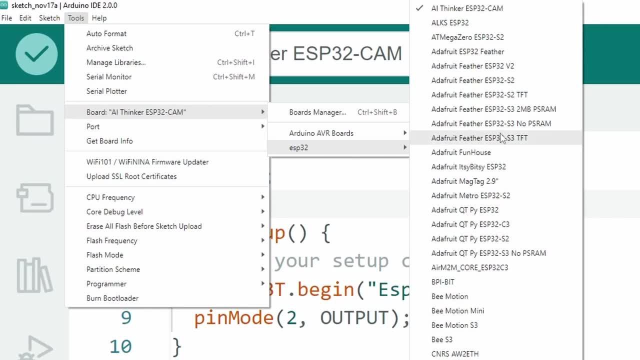 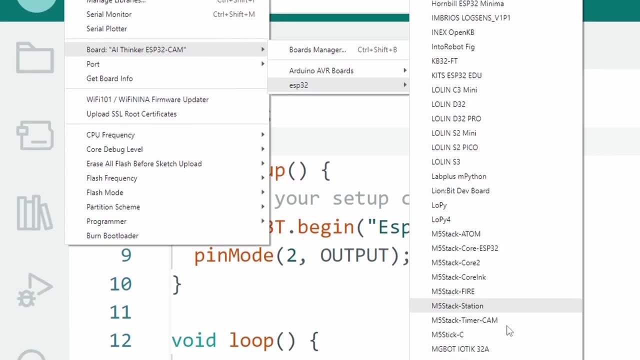 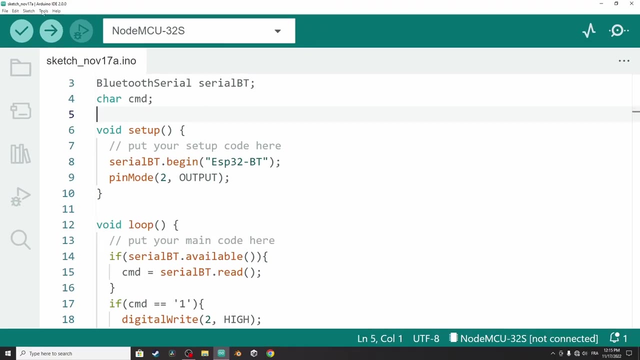 make sure to watch my first video. I've talked about that. now I can select the kind of board that I have, so let's go on and see what happens. so let's go ahead and install the Arduino IDE all the way down and search for it, and here it is: NodeMCU ESP32S. after that we select the port using. 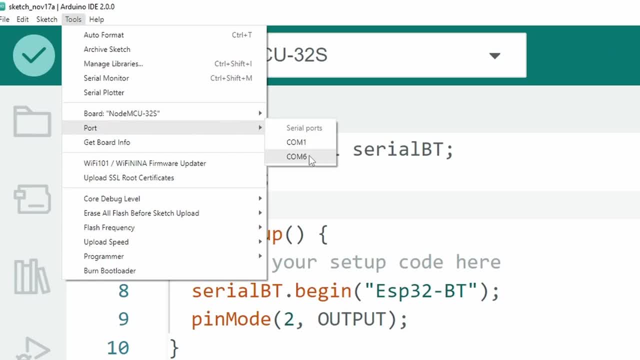 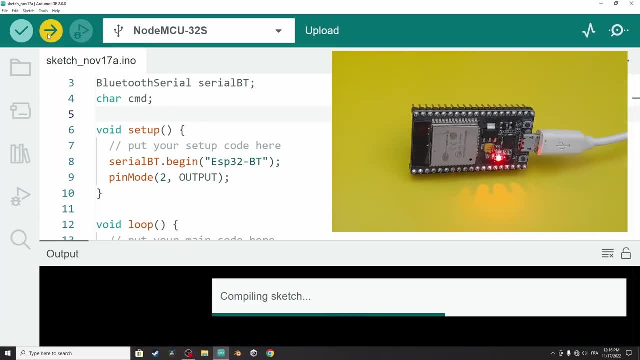 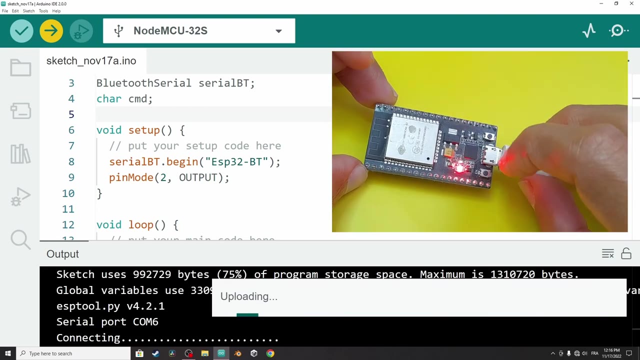 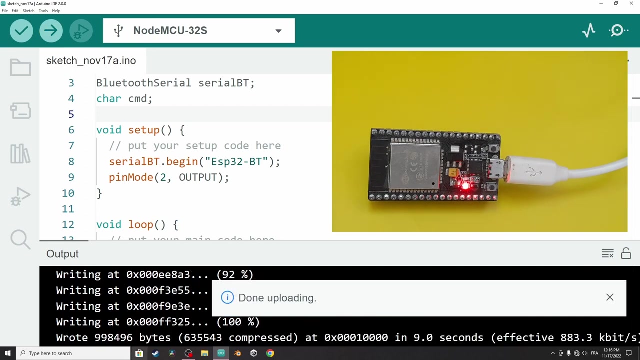 tools port- for me it is COM6- of the USB cable. then let's set upload. now it is compiling the sketch, I think everything is fine, and when you get connecting you have to hold down the boot key, which is this one. and there you go, it is uploading the code, and once it's done, we can reset our board using the RST key. 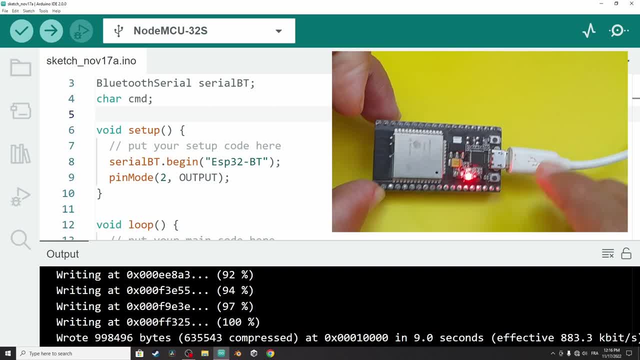 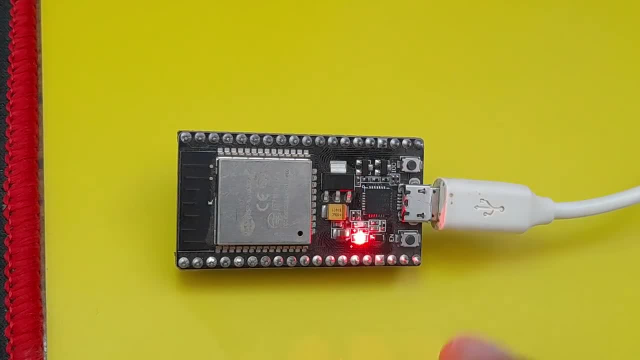 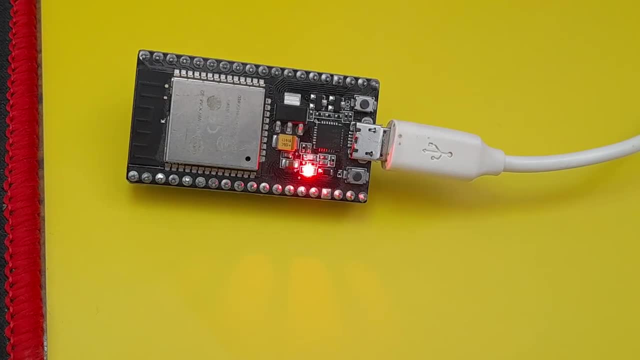 or it is called en in my board. now let's test it. but I think you are asking how we are going to send the values 1 and 0 to the Bluetooth module so that we can control the LED. basically, we can just drop it in and if every corner on the board is connected, we can see that it is already connected. 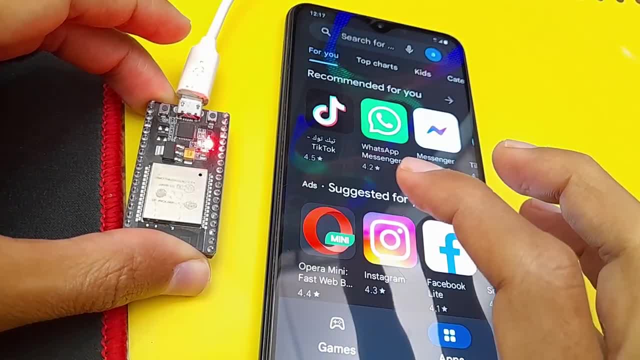 so I can't reach the stitches, but let's do it in my model. and we also have different buttons so we can change the settings over and over the mouse. we have one control panel, one on the left and one on the left for all buttons, and I want to bring the blue one in the left, since we have basically three buttons, and you can see that every one of these buttons is connected later. so I'm going to open all buttons here we can see if everything is fine. let's wrap this image. it is quite simple. right now, let's run this application and that's it. ok, so I don't have actually any. 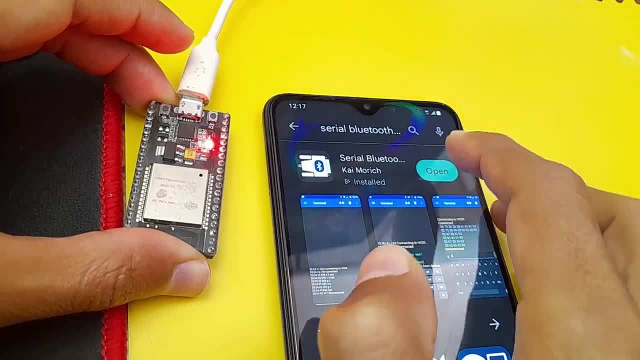 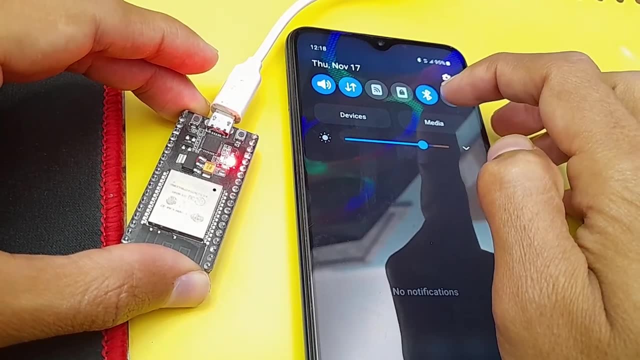 using them, so that I will be running this app. so I could also be running some tougher applications later. but this time I will be using a simple software from google play store. and let me open up google play store and search for serial Bluetooth terminal. of course you have to open up bluetooth. then let's go back to the app. under this menu we have to: